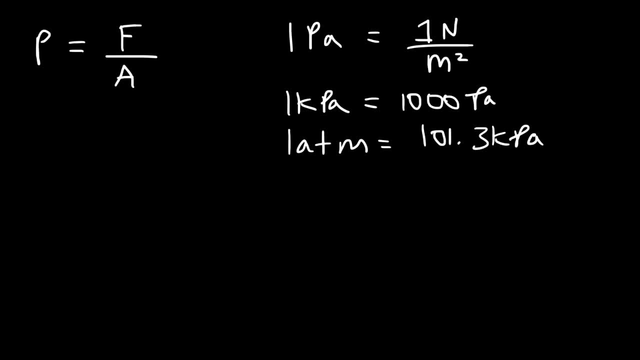 kilopascals. So those are some units that you want to keep in mind. So whenever you exert a force over a given area, that force exerts a pressure throughout that area. So pressure is simply force over area. Now what happens if you increase the area but use 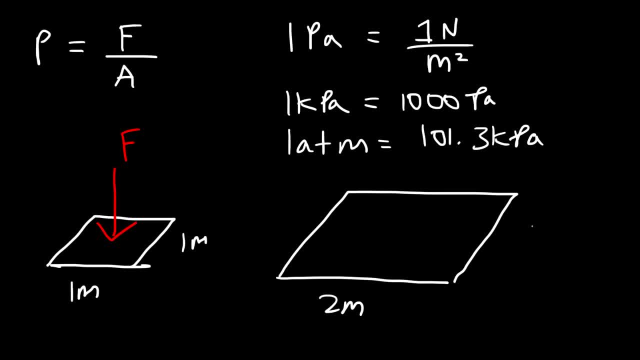 the same force. Let's say if we doubled the dimensions. Now, if you apply the same force over, let's say, a larger area, the pressure is going to be a lot less. Let's say, if we apply a force of 100. 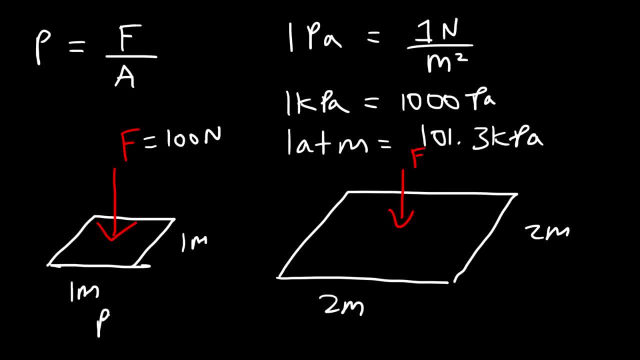 newtons. The pressure in this example is 100 divided by 1 square meter, so it's 100 pascals. In the second example, the area is 2 times 2, which is 4.. So the pressure is now a force of 100 newtons divided by an area of 4 square meters. so 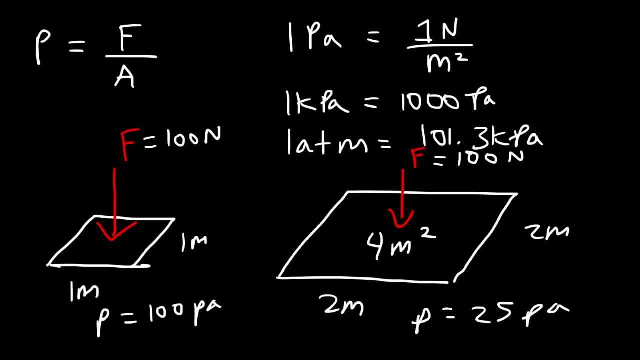 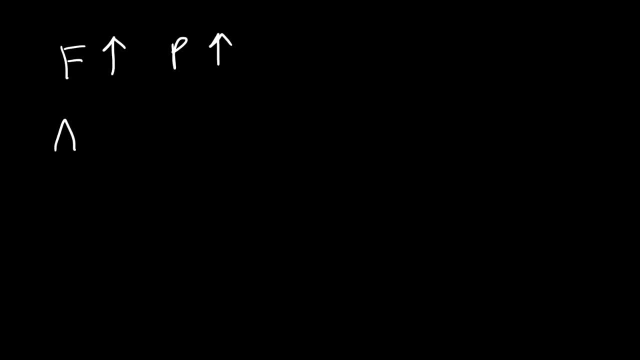 it's 25 pascals. So what you need to understand is that if you increase the force applied, the pressure increases. If you increase the area in which that force is applied, the pressure decreases. The pressure is directly related to the force, but inversely related to the 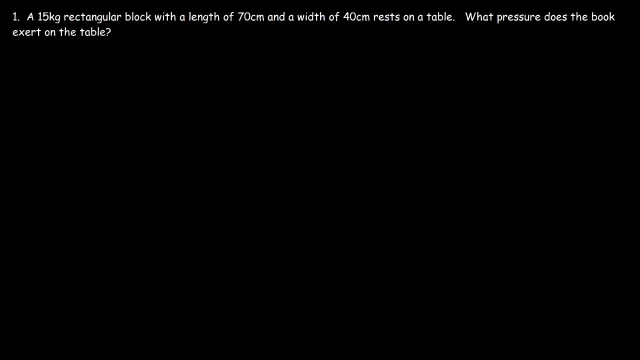 area upon which that force is applied. So if you increase the force applied, the pressure increases. Let's try this problem. A 15 kilogram rectangular block with a length of 70 centimeters and a width of 40 centimeters rests on the table. What pressure does the book exert on? 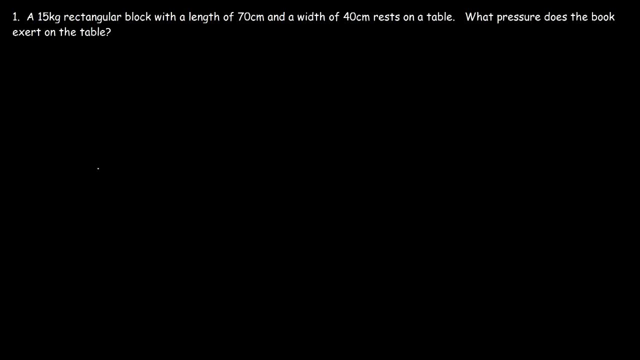 the table. So let's say this is the book And it's on the table And it's on the table. Now that book is going to exert a weight force on the table and that force is applied over 50 opens And this force, which takes a squared element, is considered a definite. 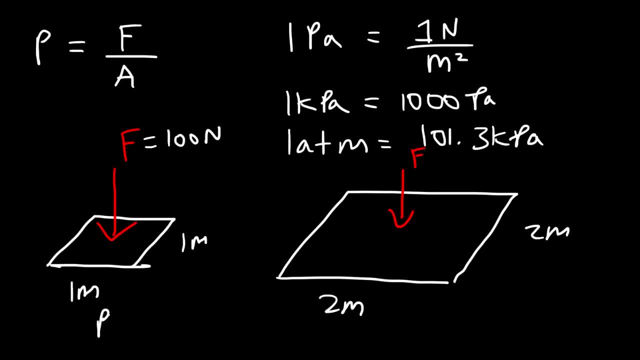 newtons. The pressure in this example is 100 divided by 1 square meter, so it's 100 pascals. In the second example, the area is 2 times 2, which is 4.. So the pressure is now. 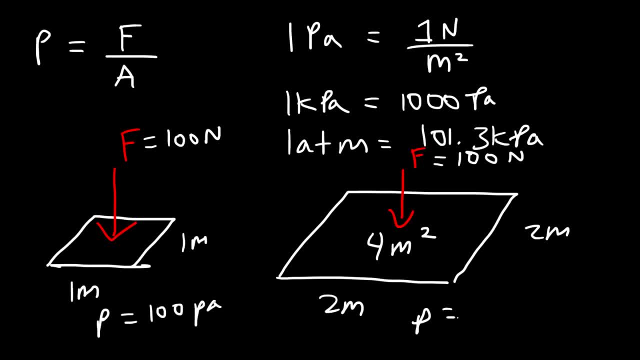 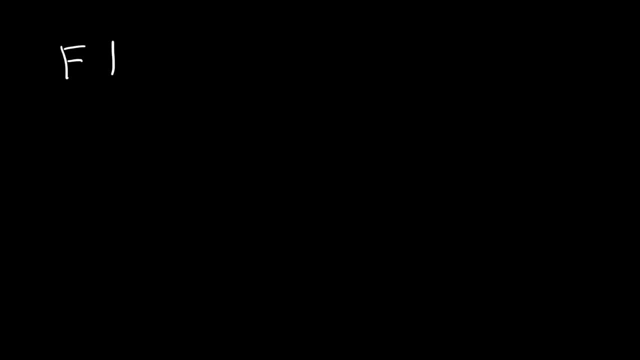 a force of 100 newtons divided by an area of 4 square meters, so it's 25 pascals. So what you need to understand is that if you increase the force applied, the pressure increases. If you increase the area in which that force is applied, the pressure decreases. 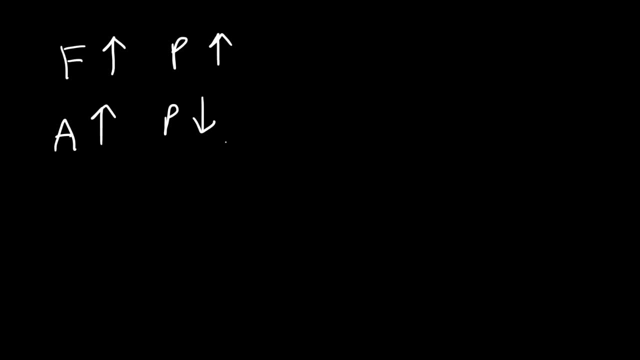 The pressure is directly related to the force, but inversely related to the area upon which that forces applied. force is applied. let's try this problem. a 15 kilogram rectangular block with a length of 70 centimeters and the width of 40 centimeters rests on the table. 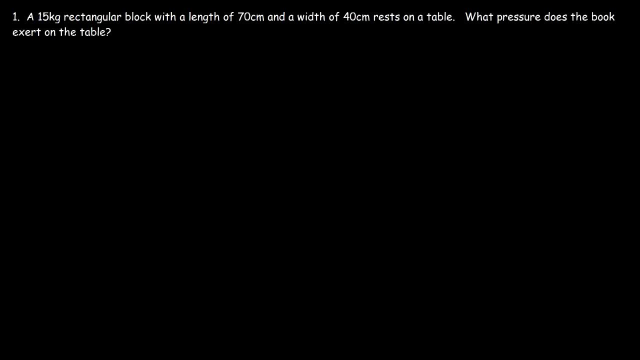 what pressure does the book exert on the table? so let's say this is the book and it's on a table. now that book is going to exert a weight force on the table and that force is applied over the, the area of the book, the bottom area. now we have a left that's 70 centimeters and 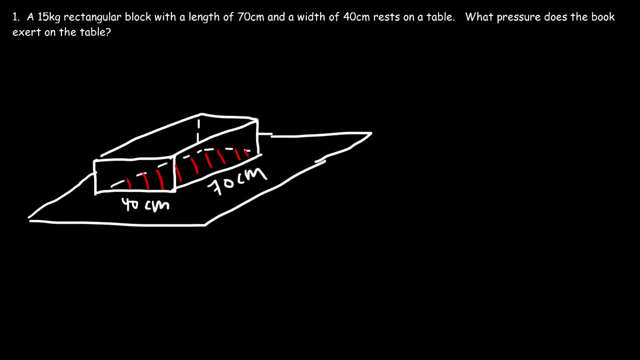 a width of 40 centimeters and we know that pressure is force divided by area and the force that the book exerts is basically the weight force of the book, which is mg. so the pressure exerted by the book is just mg divided by the area of the book. so the 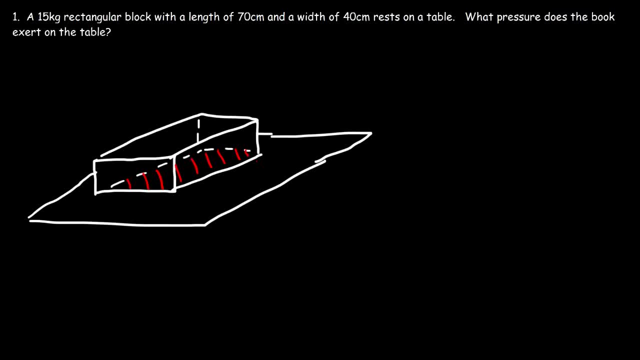 Force and void noise and void noise So that no further does this fact that gravity is the area of the book, the bottom area. Now we have a length that's 70 centimeters and a width of 40 centimeters and we know that pressure is force divided by. 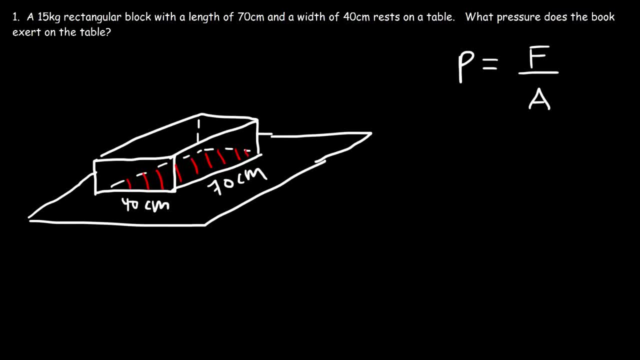 area and the force that the book exerts is basically the weight force of the book, which is mg. So the pressure exerted by the book is just mg divided by the area of the book. So the mass of the book is 15 kilograms. the gravitational 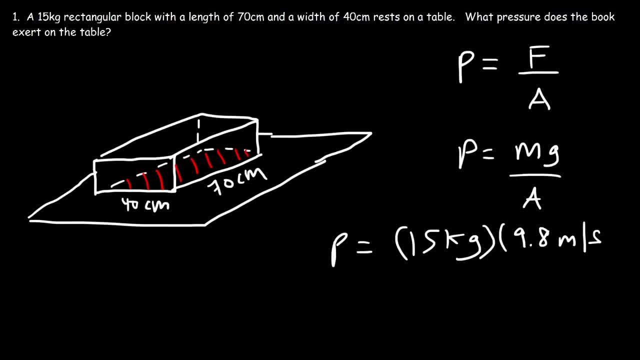 acceleration is 9.8 and the area, let's get it in square meters. so to convert centimeters to meters, divide by a hundred 70, centimeters is point seven meters and centimeters is 0.4 meters. so 15 times 9.8. so that's going to give us a force. 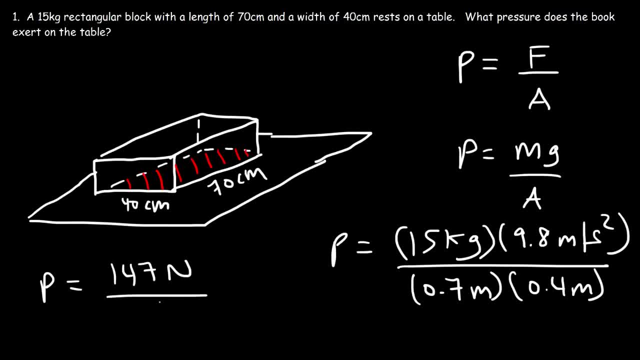 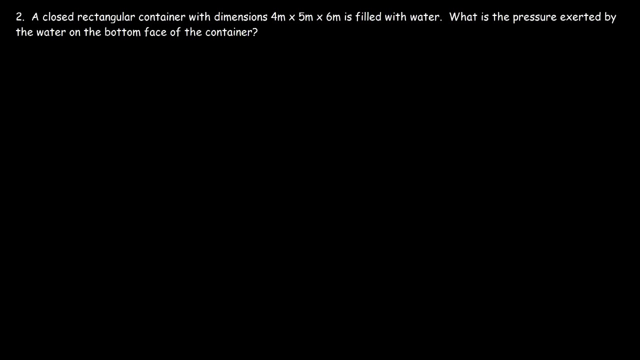 of a hundred and forty seven units and point seven times 0.4, that's going to give us an area of 0.28 square meters. so if we divide these two numbers, the pressure exerted by this book alone is 525 pascals. so this is the answer number. 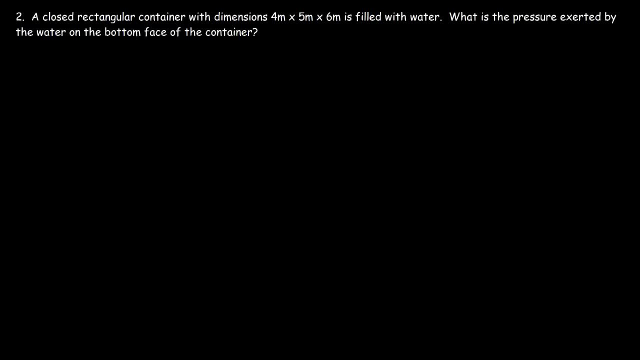 two, a closed rectangular container with dimensions four meters by five meters by six meters is filled with water. what is the pressure exerted by the water on the bottom face of the container? so let's draw a rectangular container and it's filled with water. now our goal is to find 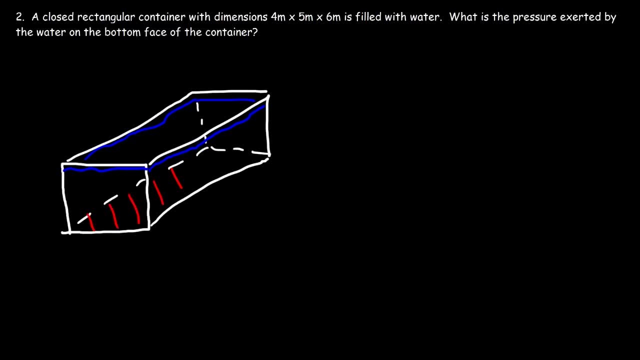 the pressure that's exerted by the weight of the water on the bottom surface of the cube. so how can we do that? well, we know pressure is force over area and keep in mind the density of water, if you're wondering, is a thousand kilograms per cubic meter. 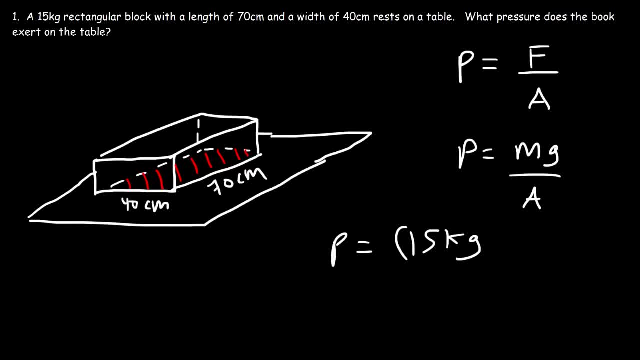 mass of the book is 15 kilograms, the gravitational acceleration is 9.8 and the area. let's get it in square meters. so to convert centimeters to meters, divide by 100: 70 centimeters is .7 meters and 40 centimeters is .4 meters. 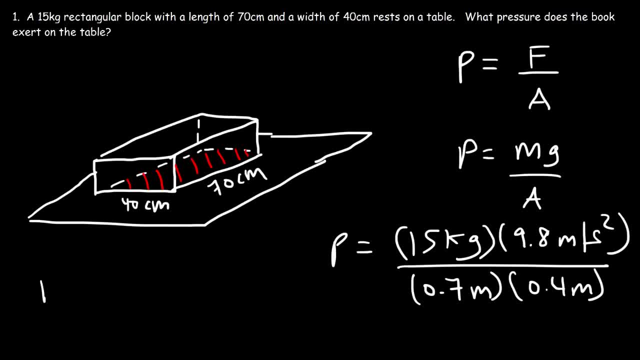 so 15 times 9.8, so that's going to give us a force of 147 units, and .7 times .4, that's going to give us an area of .28 square meters. so if we divide these two numbers, the pressure exerted by this book alone is 525 pascals. so this is the 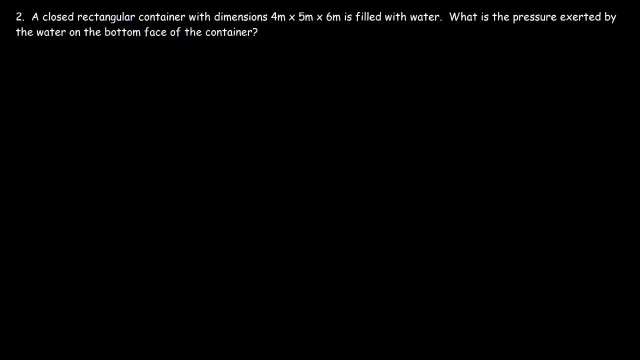 answer Number two. a closed rectangular container with dimensions four meters by five meters by six meters is filled with water. What is the pressure exerted by the water on the bottom face of the container? So let's draw a rectangular container and it's filled with water. 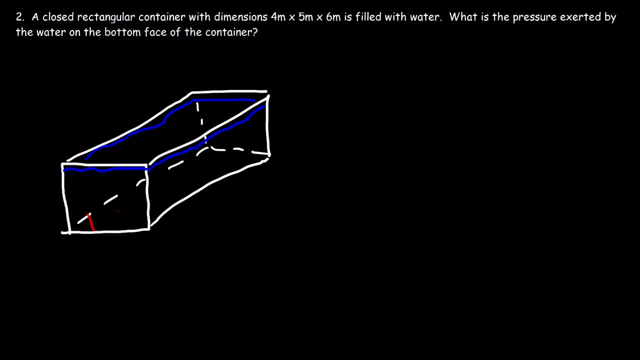 Now our goal is to find the pressure that's exerted by the weight of the container Under the water, on the bottom surface of the cube. So how can we do that? Well, we know pressure is force over area, And keep in mind the density of water, if you're wondering, is a thousand kilograms per cubic. 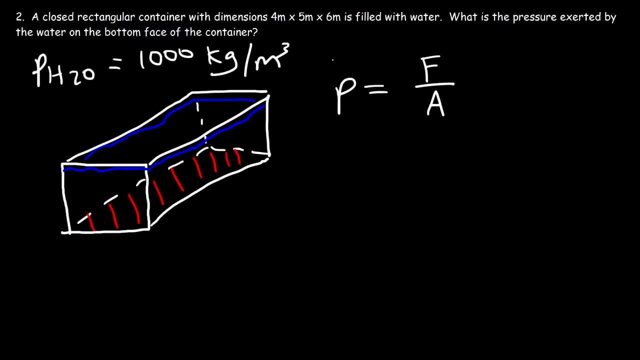 meter. Now the force Is the weight of the water, which is mg, And we don't have the mass of the water. However, we know that density, which is rho, is mass over volume. Don't confuse this with pressure. So the mass of the fluid, if we multiply both sides by v, is density times volume. 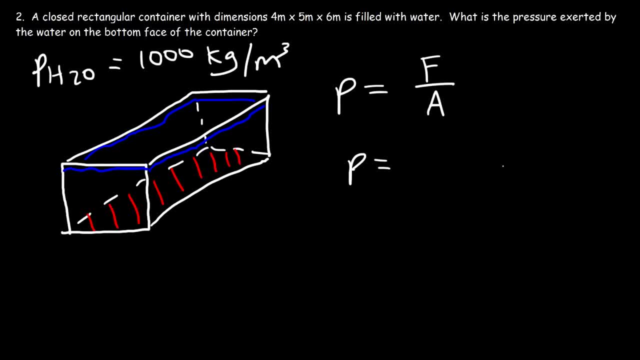 now the force is the weight of the water, which is mg, and we don't have the mass of the water. however, we know that density, which is row, is mass over volume. don't confuse this with pressure. so the mass of the fluid, if we multiply both sides by V, is: 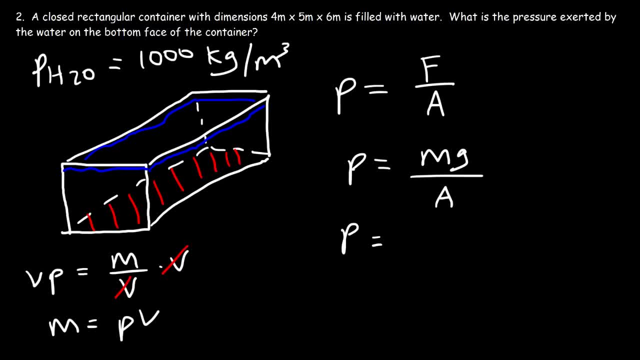 density times volume. so the pressure of the fluid is going to be the mass which is density times volume and then times gravitational acceleration, divided by the area. now the volume of, let's say, this rectangular prism is the left times the width times the height. let me write that somewhere. 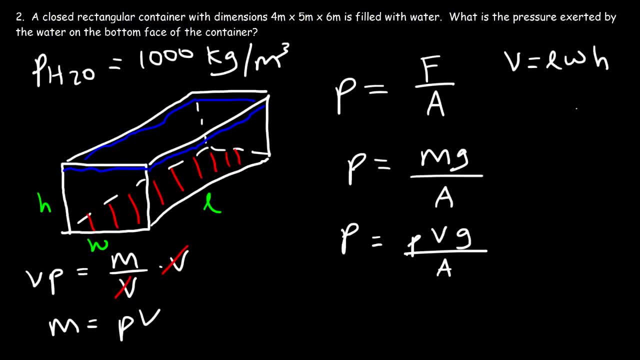 now the left times the width will give us the area of the bottom surface. or rather, I'm just going to replace volume with left times, width times, height, and the area of the bottom surface is just the left times the width. so we could cancel L and W, so the 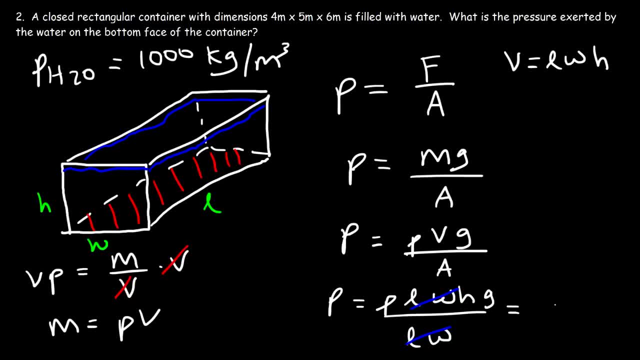 pressure that's due to the weight of the water alone. it's going to be the density of the fluid times the gravitational acceleration times the height of the fluid. so here it is. this is the equation that you want to keep in mind when dealing with the pressure due to a fluid. so we know the density of water is a thousand. 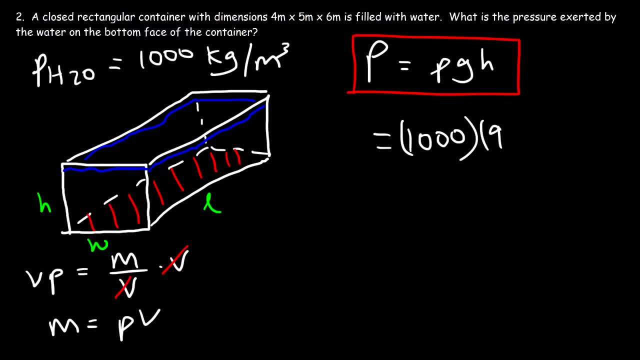 kilograms per cubic meter. we have the gravitational acceleration- it's 9.8, and the height of the fluid. now let's say the first one is the length, the second is the width, so the height we're going to say it's 6 meters in this example. 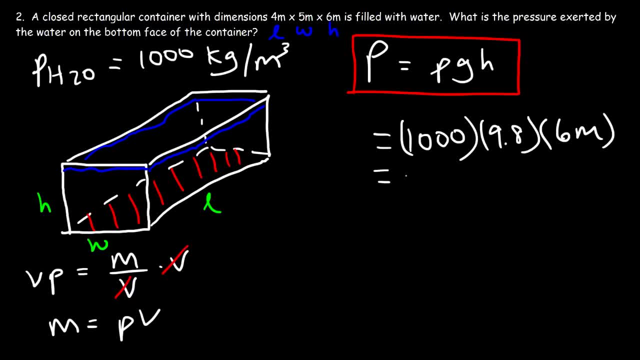 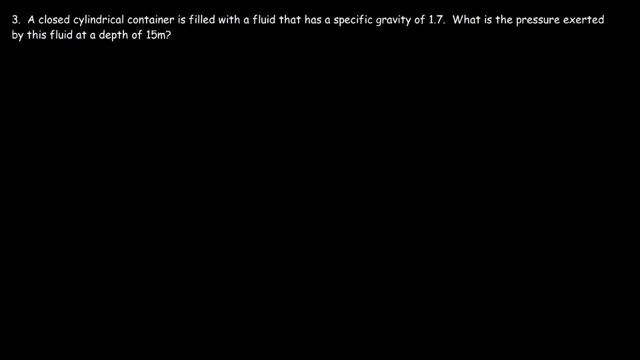 So it's going to be 1,000 times 9.8 times 6.. So the pressure is 58,800 pascals. So that's the pressure due to the weight of the water alone. Number three: a closed cylindrical container is filled with a fluid that has a specific 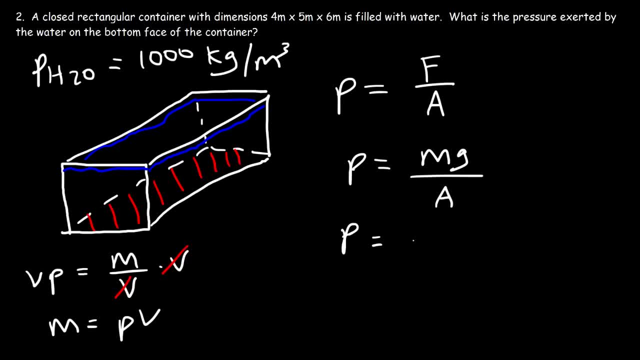 So the pressure of the fluid Is going to be the mass, which is density times volume and then times gravitational acceleration, divided by the area. Now the volume of, let's say, this rectangular prism is the length times the width, times the height. So let me write that somewhere. 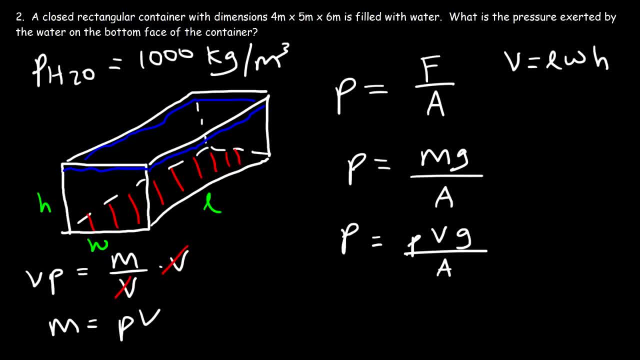 Now the length times the width will give us the area Of the bottom surface. Or rather, I'm just going to replace volume with length times width times height, And the area of the bottom surface is just the length times the width. So we could cancel L and W. 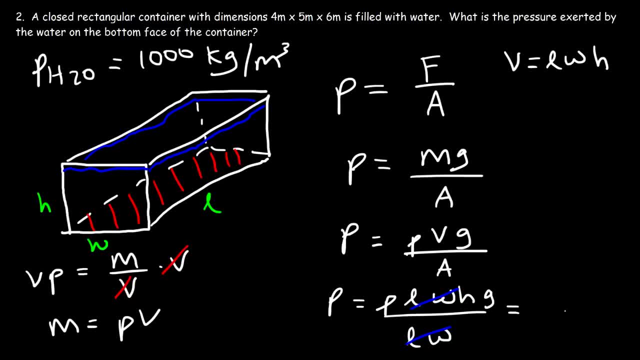 So the pressure that's due to the weight of the water alone Is going to be The density of the fluid times the gravitational acceleration times the height of the fluid. So here it is. This is the equation that you want to keep in mind. 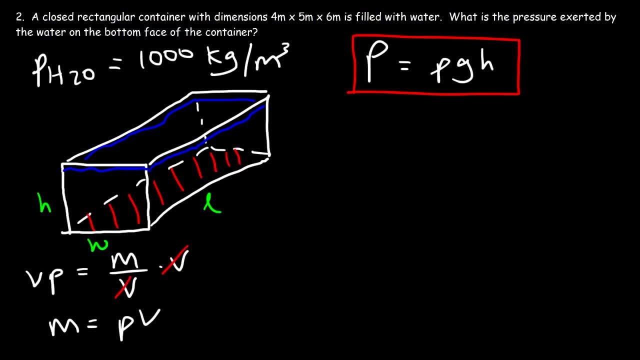 When dealing with the pressure due to a fluid. So we know the density of water is 1000 kilograms per cubic meter. We have the gravitational acceleration: It's 9.8.. And the height of the fluid? Now let's say the first one is the length. 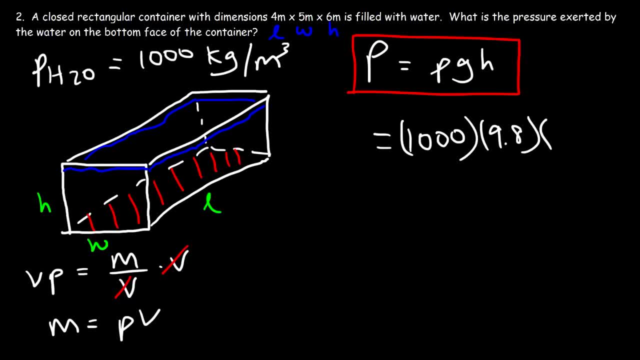 The second is the width, So the height. We're going to say it's 6 meters in this example. So it's going to be 1000 times 9.8 times 6.. So the pressure is 58,800 pascals. 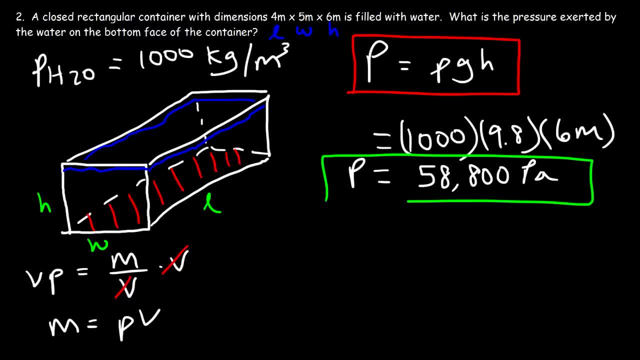 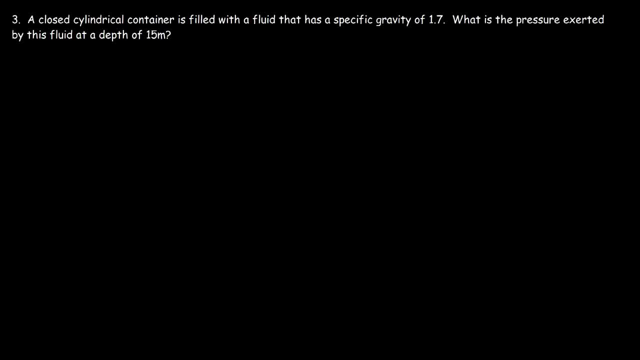 So that's the pressure due to the weight of the water alone. Number three: A closed cylindrical container is filled with a fluid that has a specific gravity of 1.7.. What is the pressure exerted by this fluid at a depth of 15 meters? 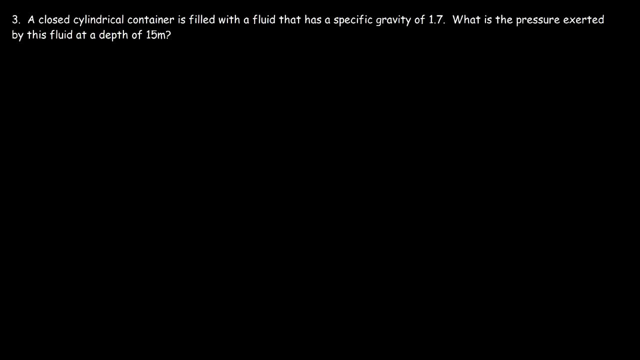 gravity of 1.7.. What is the pressure exerted by this fluid at a depth of 15 meters? So let's say: this is the cylindrical container and it's, It's closed and it's filled with some fluid. So at a depth of 15 feet- I mean not feet but 15 meters- let's say at this point we 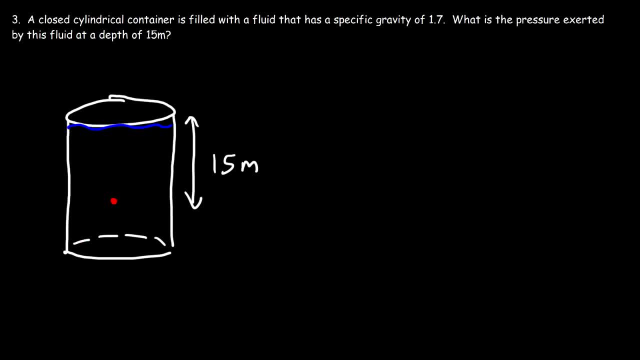 want to know what's the pressure exerted at that depth. So we can use this equation: The pressure is equal to the density times gravity times the height. So if you have a fluid and you want to find the pressure exerted by the fluid alone at 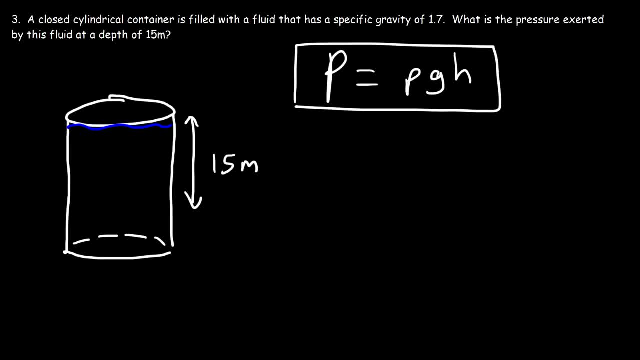 a certain depth. this is the equation that you can use. Now we need to know what the density of this fluid is, and we're given that specific gravity. The specific gravity is the density of the substance, in this case, the density of fluid. 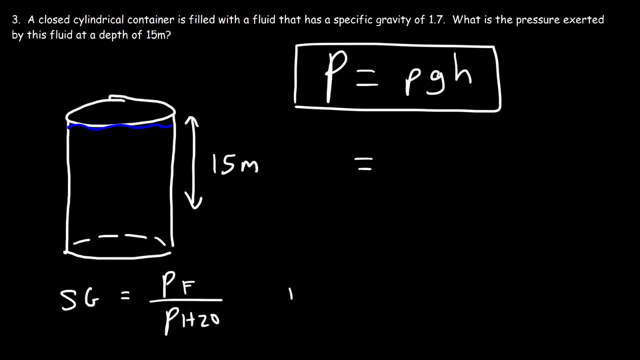 relative to the density of water. So the density of the fluid is going to be the specific gravity and the density of the fluid is going to be the density of water. So we have a specific gravity of 1.7, and the density of water is 1,000 kilograms per cubic meter. 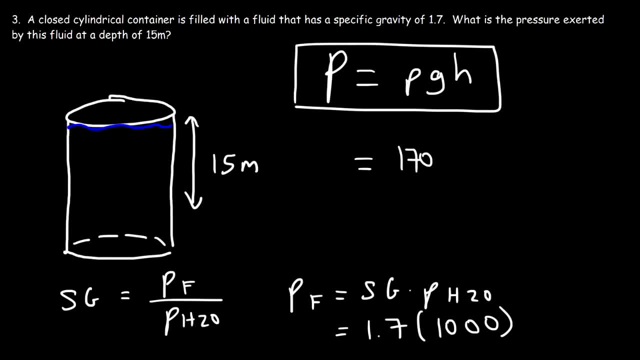 So the density of the fluid is 1,700 kilograms per cubic meter. Now we have the gravitational acceleration and the depth is 15 meters. So it's 1,700 times 9.8 times 15.. So the pressure exerted by this fluid at a point where it's 15 meters deep is 249,900 pascals. 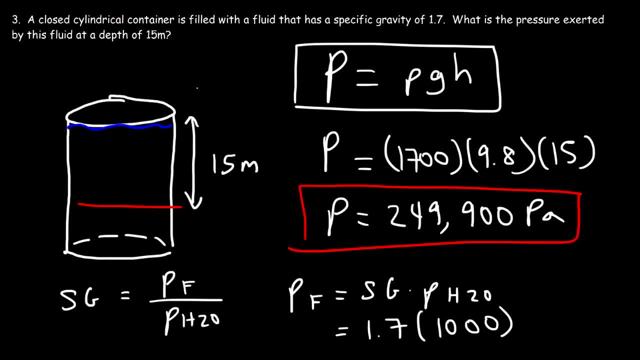 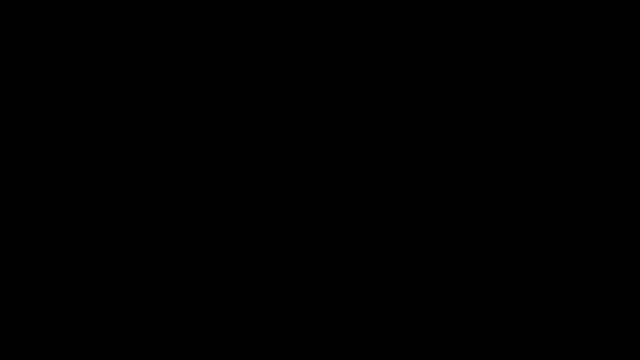 And if you divide that by 1,000, you could say it's about 249.9 kilopascals. So we have a specific gravity and the density of the fluid is 1,000 kilograms per cubic meter.